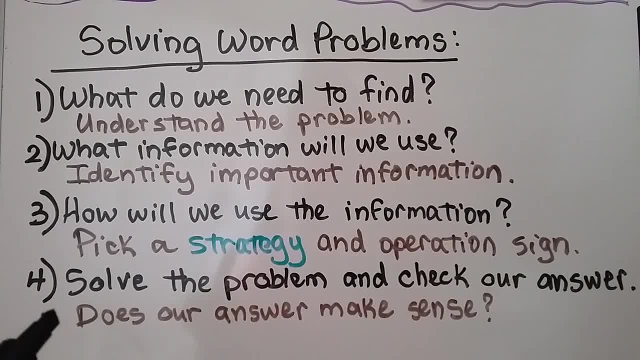 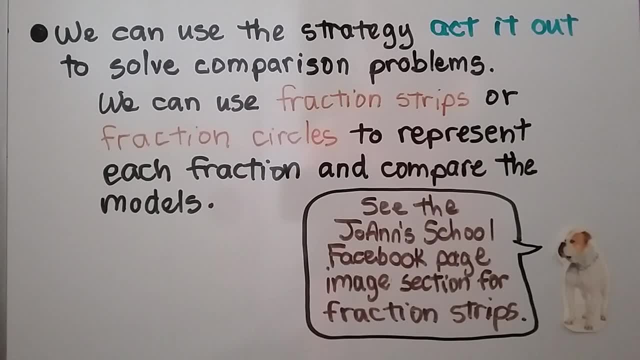 divide. Then we're going to solve the problem and check our answer. We want to know if our answer makes sense. We can use the strategy, act it out to solve comparison problems. We can use fraction strips or fraction circles to represent each fraction and compare the models we can compare. 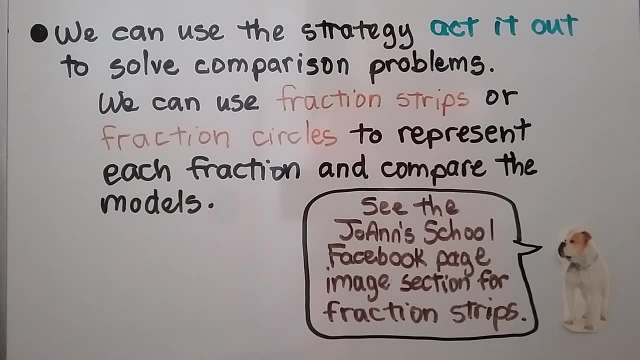 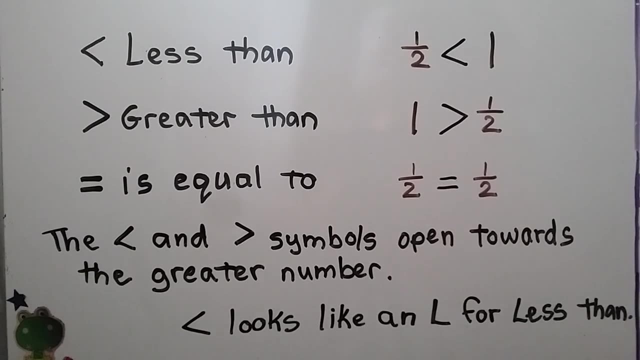 the size of the models to each other and you can go to the joann school facebook page image section for fraction strips that you can print, copy paste and cut out and use for your homework. so remember, this is the sign right here. for less than, do you see it right here? 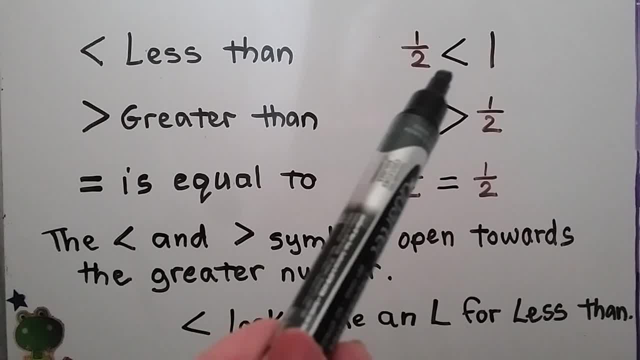 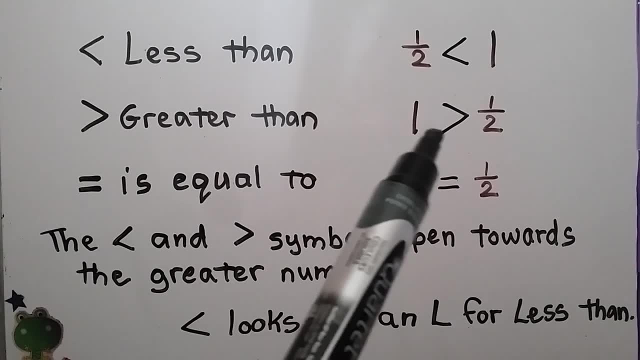 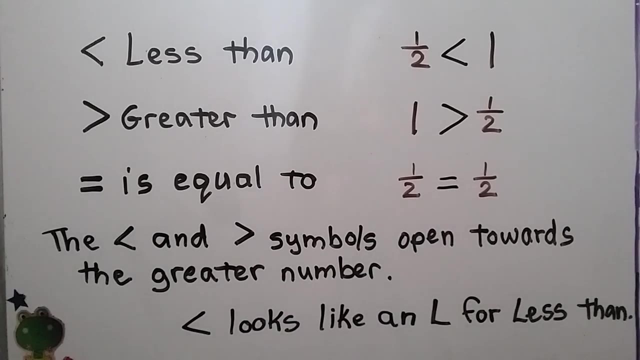 and a half of something is less than a whole thing, isn't it? so we have a less than sign there. this is the greater than sign. one is greater than half and of course, you know, is equal to a half is equal to a half, and the less than and greater than symbols open towards the greater. 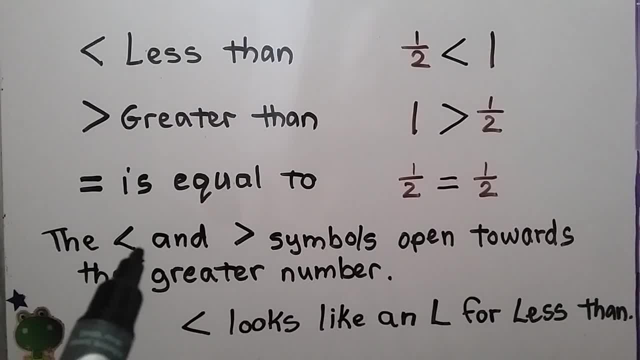 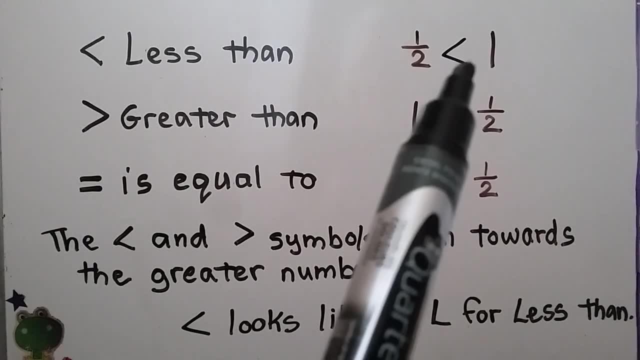 number. so whichever is the greater number, that's the side that's open, more like here: one is greater, so the big side is open to the one, and on this one the one is greater, so the big side is open to the one. see that, and this less than symbol kind of looks like a crooked l, doesn't it? 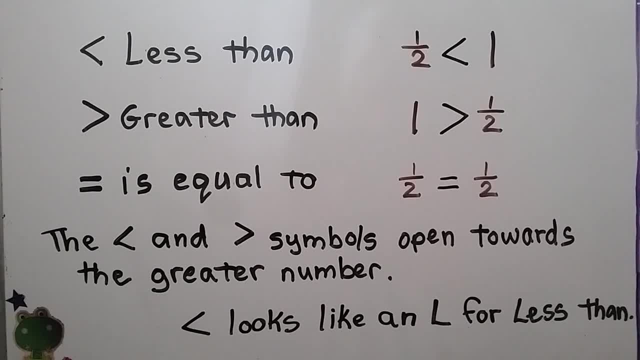 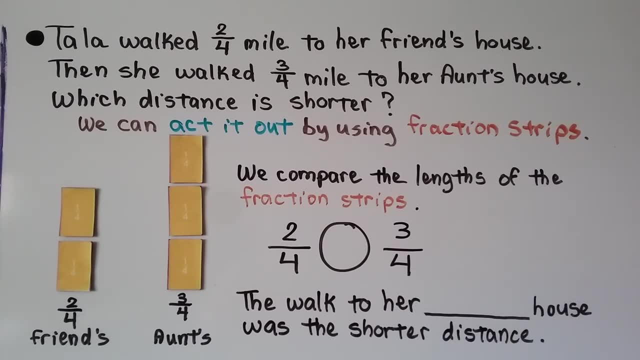 for less than like the l in less, talla walked two-fourths mile to her friend's house. then she walked three-fourths mile to her aunt's house, which distance is greater than the other one, and the distance is shorter and we can act it out by using fraction strips, so we need to use 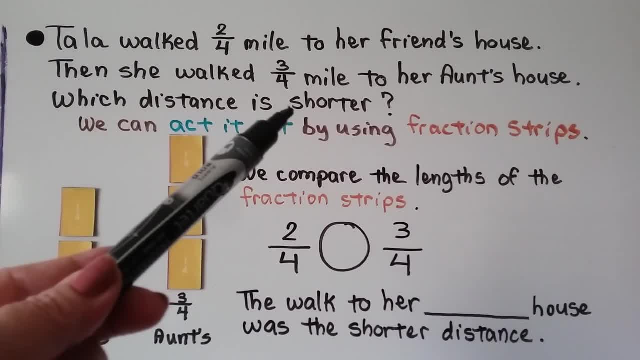 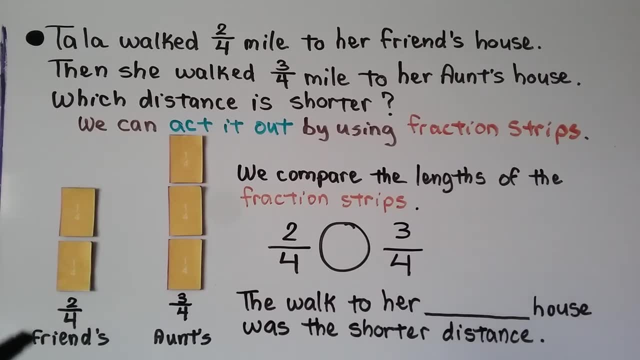 two-fourths and three-fourths. we need to know that they're asking us which one is shorter. we have two one-fourth fraction strips, so that's two-fourths. that's the distance she walked to her friend's house, and we have three one-fourth fraction pieces. that's the distance she walked to. 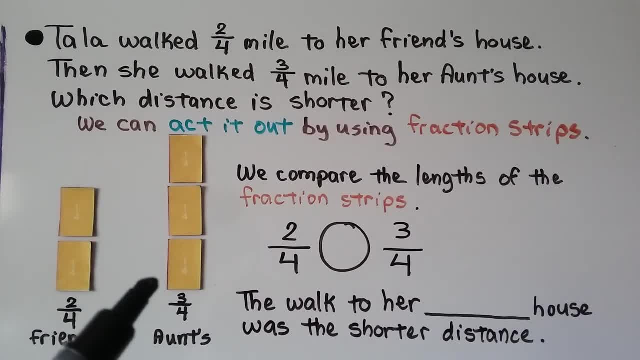 mile and we can see the three-fourths is much bigger, isn't it? it's another fourth, isn't it? so two-fourths is less than three-fourths because the three-fourths is the greater fraction. we have the big open part facing the greater fraction. so the walk to her. 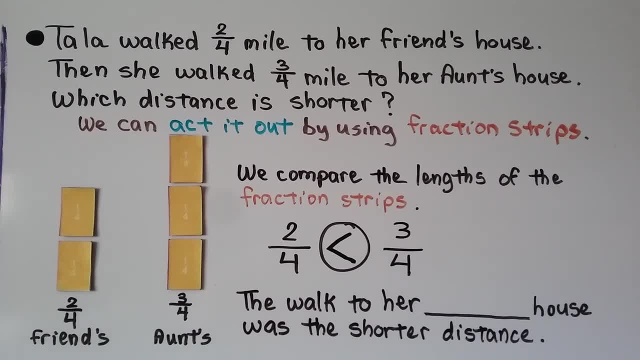 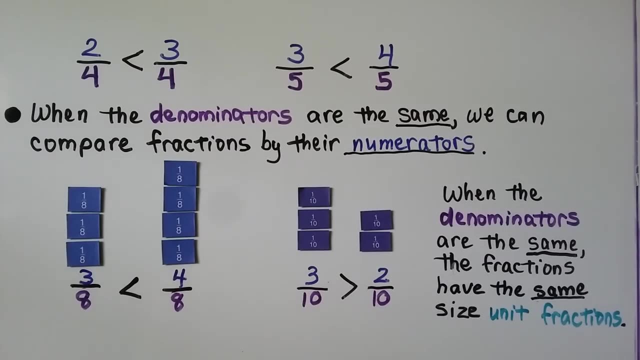 the walk to her friend's house was the shorter distance. it's very important that we make sure we answer what it was asking: which distance is shorter- the two-fourths to her friend's house? when the denominators are the same, we can compare fractions by their numerators. this has got a denominator of four, and so does this one. 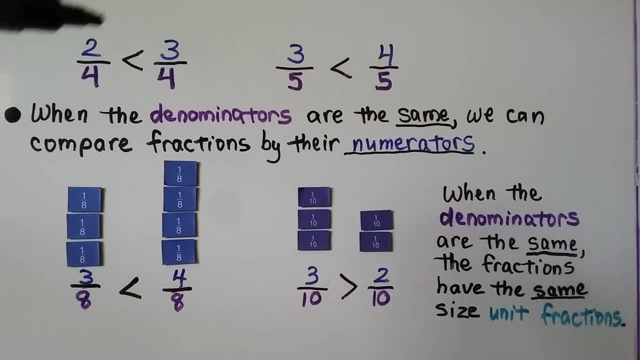 so we can just look at the numerator two and three. which one's bigger? three, that means three. 3 fourths is greater than 2 fourths. See: 2 fourths is less than 3 fourths. Here they both have a denominator of 5, so we can use the numerator to compare them. 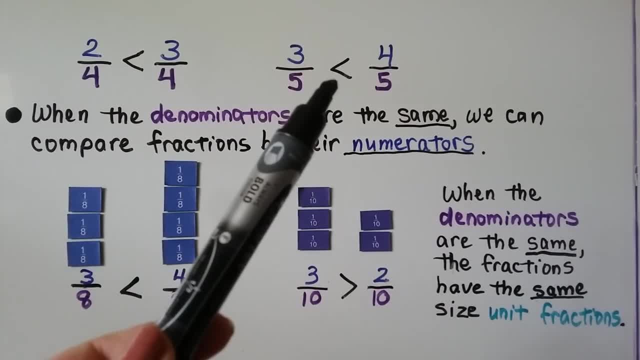 3 is less than 4, so 3 fifths is less than 4 fifths. So when the denominators are the same, the fractions have the same size: unit fractions. Remember, a unit fraction has a 1 for a numerator. 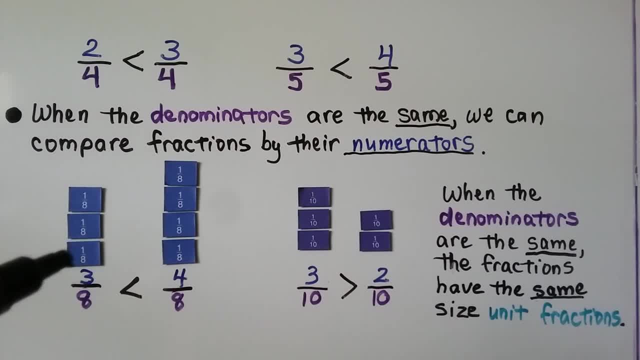 So here we have a unit fraction, a unit fraction and a unit fraction. It's 1 eighth, 1 eighth and 1 eighth, That's 3 eighths. The denominators are the same, so we use the numerators to compare them. 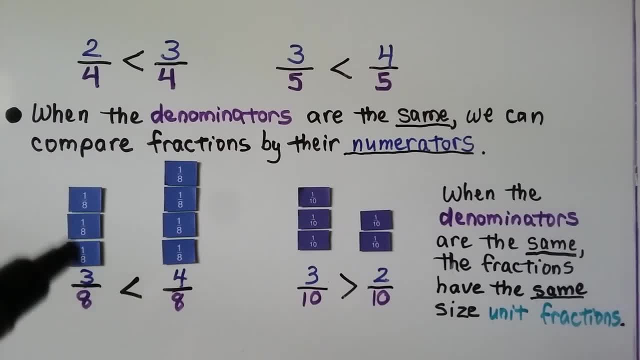 3 is less than 4.. See, we have 3 of them here and 4 of them there. That's because the denominators are the same. Here we've got 1 tenth unit fractions. We've got 3 of them here and 2 of them here. 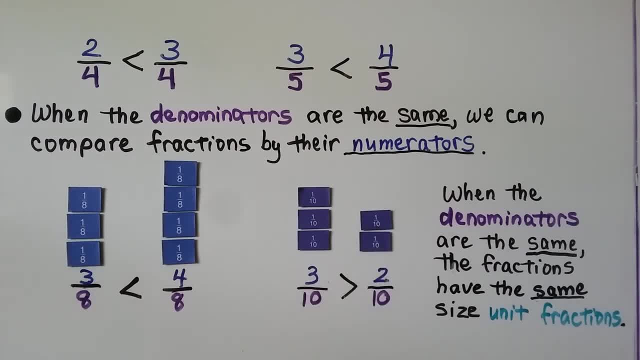 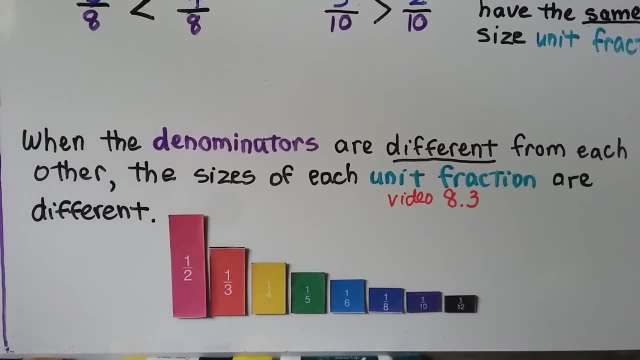 So 3 tenths is greater than 2 tenths. We'll talk about this more in the next lesson too. When the denominators are different from each other, the sizes of each unit fractions are different. So here we have a denominator 2, and here we have a. 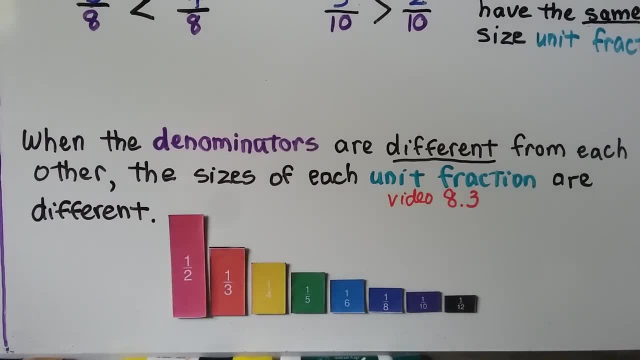 denominator 3.. See how the unit fractions are different sizes. And when the denominator is 4, it's a different size than that one. And do you notice that the larger the denominator number becomes, the smaller the piece is? Do you see that When we get to 1 twelfth, it's a very tiny little piece, but one half. 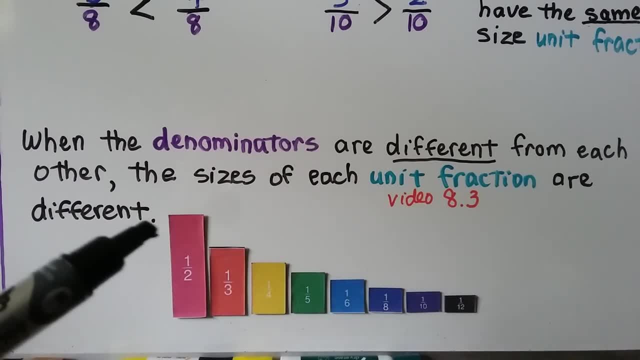 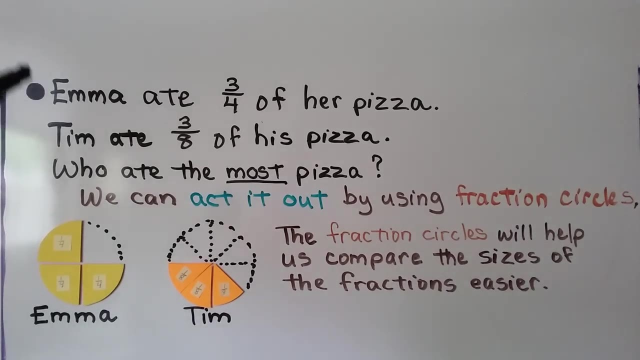 that has a 2 for a denominator is a much bigger piece. That's because the whole thing was only cut into two parts, Where this whole thing was cut into 12 parts and that's just one of them. Emma ate 3 fourths of her pizza. 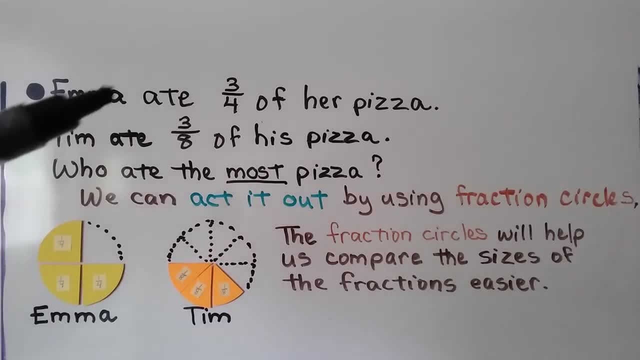 Tim ate 3 third's eighths of his pizza. So they each had their own pizza, didn't they Who ate the most pizza? We can act it out by using fraction circles. So these are fraction circles, A whole. one would make a whole circle. See, Emma has a fourth. a fourth. 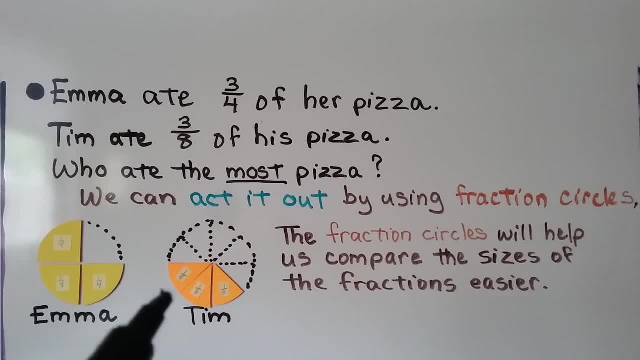 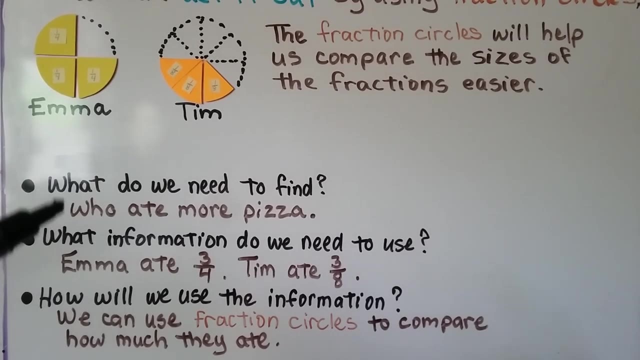 and a fourth, That's three fourths that she ate, And Tim has an eighth, an eighth and an eighth for three eighths that he ate, And the fraction circles will help us compare the sizes of the fractions easier. So what do we need to find? We 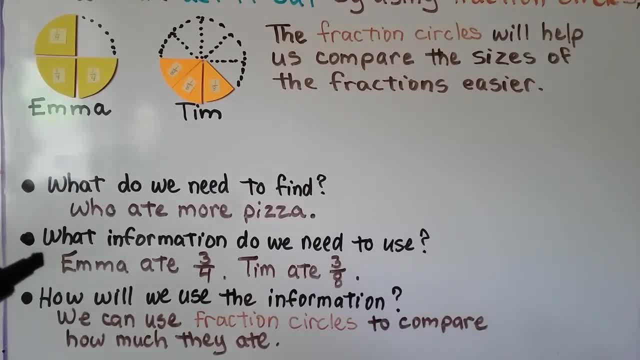 need to find who ate more pizza, And what information do we need to use? We need the information that Emma ate three fourths and Tim ate three eighths. And how will we use the information? We can use fraction circles to compare how much. 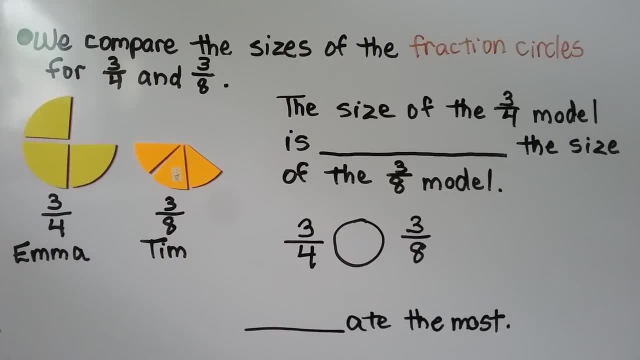 they ate. We compare the sizes of the fraction circles for three, eighths and a fourths. We can use the information that the three-fourths and three-eighths And the size of the three-fourths model is: it's larger, it's. 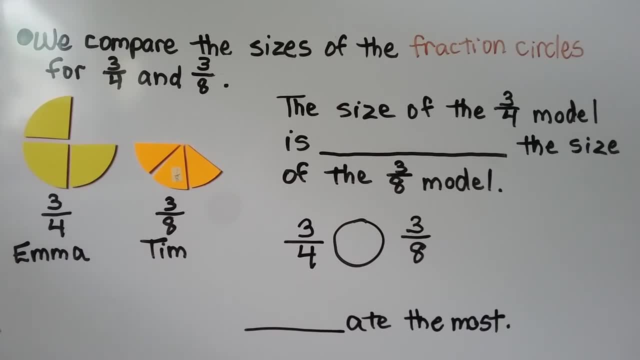 greater than the size of the three-eighths model, isn't it? There's a lot more pizza here. If that's how much she ate, that's more than that one, isn't it? So it's greater than the size of the three-eighths. 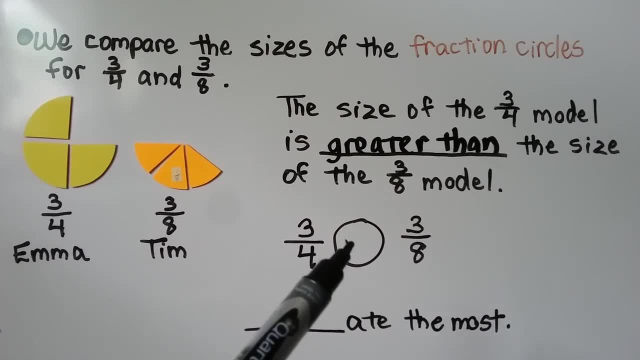 model. We can put a greater than sign here that three-fourths is greater than three-eighths. So who ate the most? Emma? Emma ate the most, didn't she? Three-fourths is greater. Maybe they're saving it for later, The rest of it. 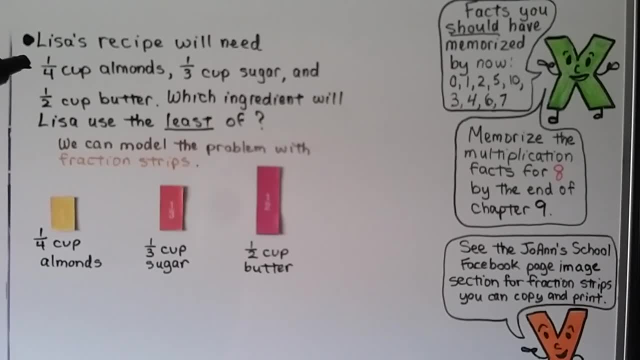 Lisa's recipe will need one-fourth cup almonds, one-third cup of sugar and one-third cup of water, One-half cup sugar and one-half cup butter. So which ingredient will Lisa use? the least of that means the smallest amount, And the first thing we need to notice is that it's cup, cup and cup. 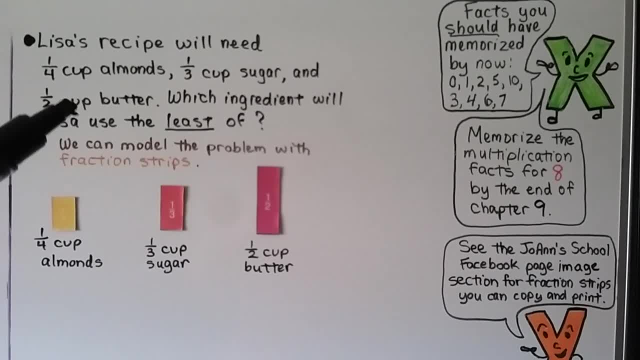 Because then we're comparing the same type of measurement. Because what if that said one-fourth teaspoon? Well, a teaspoon is way smaller than a cup, isn't it? So this is one-fourth cup, one-third cup, one-half cup. 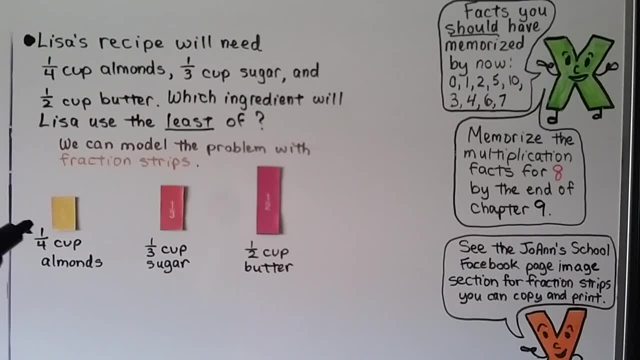 We can model the problem with fraction strips. One-fourth cup, that's the almonds, it would be a one-fourth fraction piece. One-third cup sugar would be a one-third fraction piece And one-half cup butter. we could use a half. 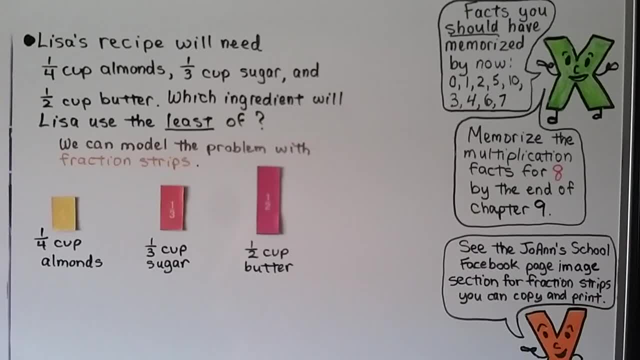 fraction piece. Then we can just look at them. And which ingredient will Lisa use the least of The smallest amount of? If you said almonds, you're right. That's the smallest fraction of the three Out of one-fourth. one-third and one-half one-fourth is the smallest fraction, It's the least. 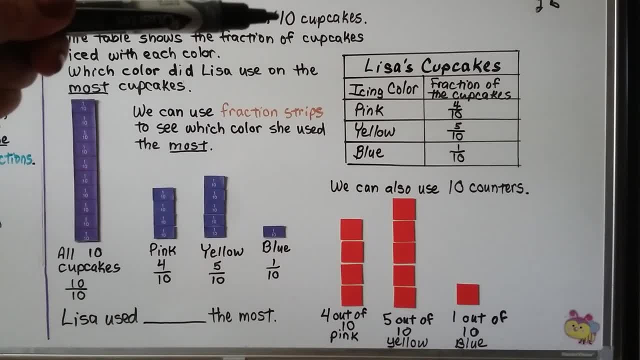 Lisa is putting icing on ten cupcakes And The table shows the fraction of cupcakes iced with each color. Which color did Lisa use on the most cupcakes? So let's take a look at our frequency table here. Here it's Lisa's cupcakes. 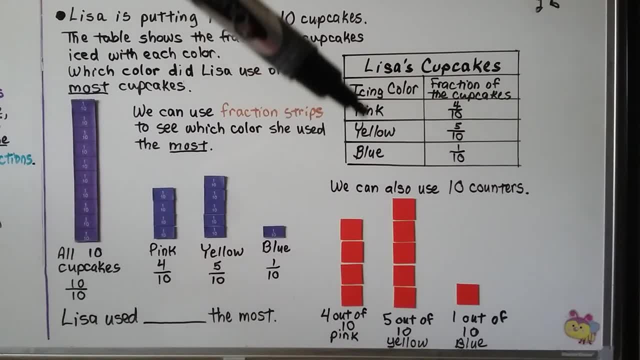 We can see this is icing color of pink, yellow or blue and the fraction of the cupcakes. There's 10 cupcakes, so 4 tenths, which means 4 out of the 10, was pink 5 tenths, which. 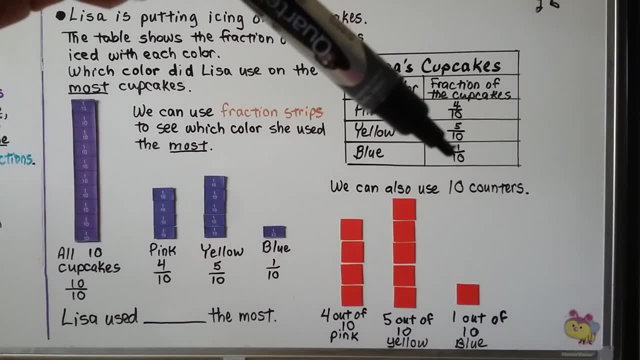 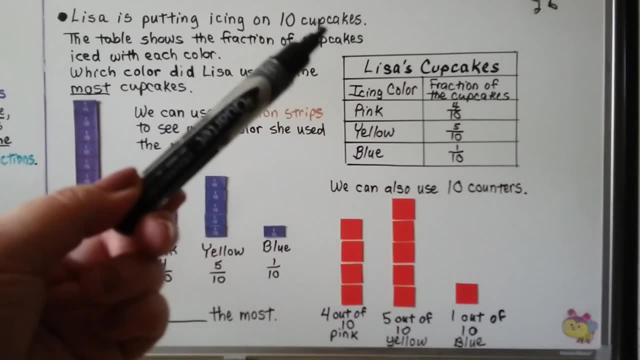 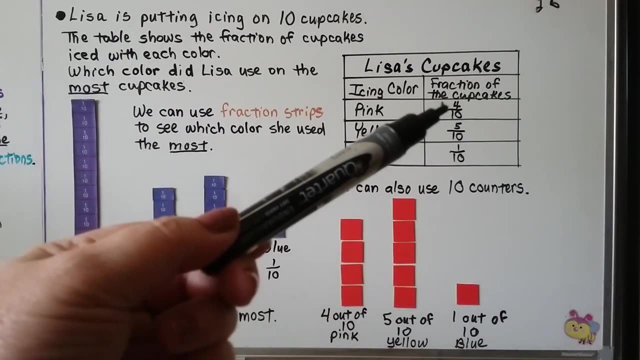 means 5 of the 10 were yellow and 1 tenth, which means 1 of the 10 was blue. If we look at these fractions- because 10 cupcakes is the whole thing right, It's all of them that would fit in the box that she's making of cupcakes. 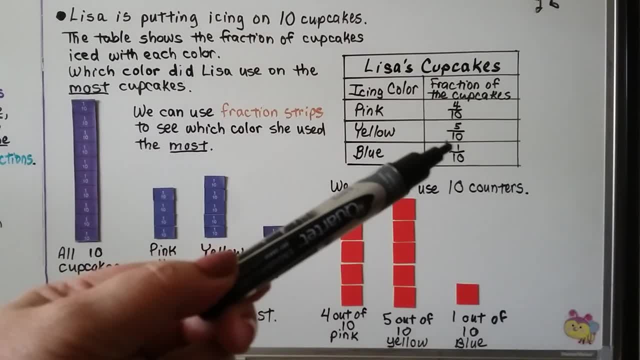 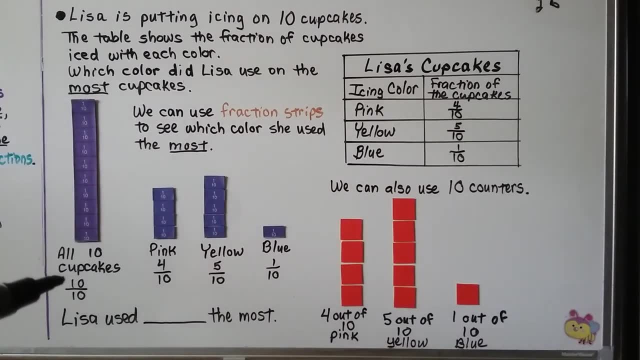 We add the numerator 4 plus 5, which is 9, plus 1 more is 10, and that equals all 10 cupcakes, 10 tenths, one whole thing of 10 cupcakes. see So here's one whole and it's split into unit fractions of 1 tenth, and there's 10 of them. 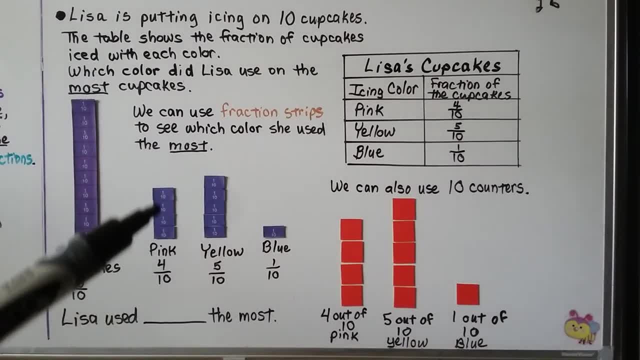 For the pink icing she had 4 tenths. That means she had 4 of these, That's 4 out of 10 cupcakes were pink. For the yellow icing it was 5 of the 10, it was 5 tenths. 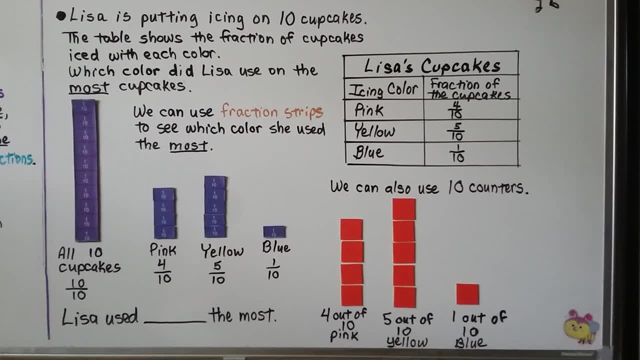 And for the blue it was only 1 tenth, 1 of the 10.. So we can look at these three and tell which one she used the most. It was yellow, wasn't it? Lisa used yellow the most. Did we answer the question? 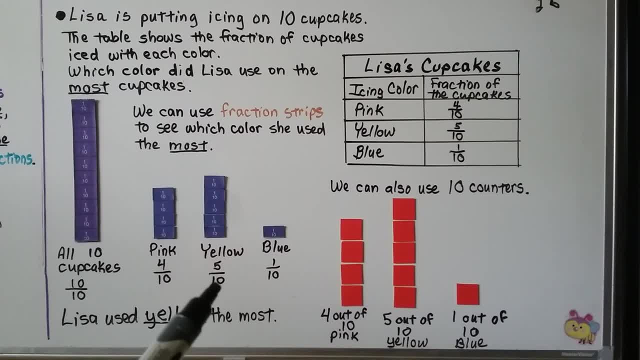 Which color did Lisa use the most? Yes, we did. Does it make sense? Yes, because that has the longest fraction bar, doesn't it? Now, we also could have used counters. We could have used 10 counters because there's 10 cupcakes and we could have pretended that. 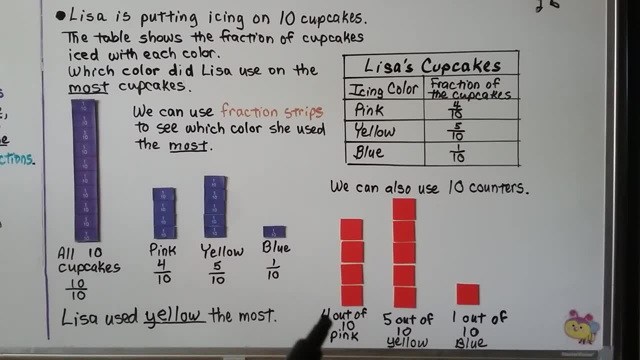 each counter was a cupcake and 4 tenths, or 4 out of 10, were pink. so we have 4 counters. 5 tenths, or 5 out of 10, were yellow. so we used 5 counters and 1 tenth- 1 out of 10. 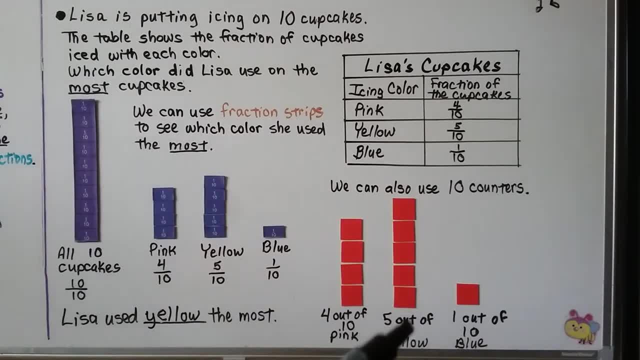 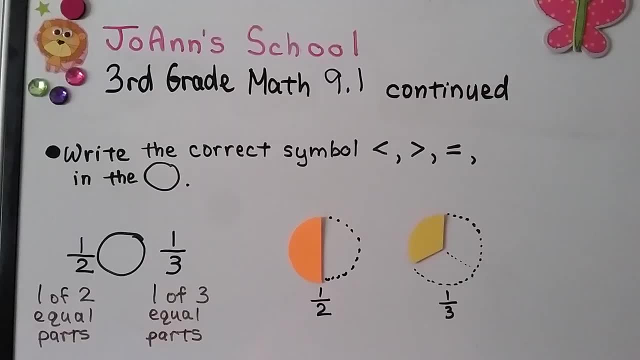 was blue. We have 1 counter And we can see that we have more counters for the yellow, so Lisa used yellow the most. We can write the correct symbol. We can write less than greater than equal to in the circle. 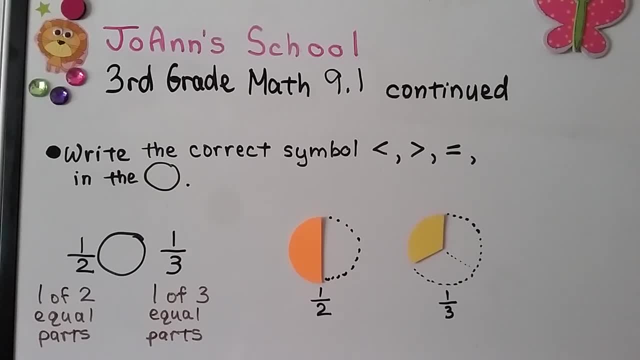 So we're going to compare 1 half and 1 third. One half means 1 of 2 equal parts. One third means 1 of 3 equal parts. Well, One half would be 1 of 2 equal parts. See, there would be 2 parts and we have 1 of them. 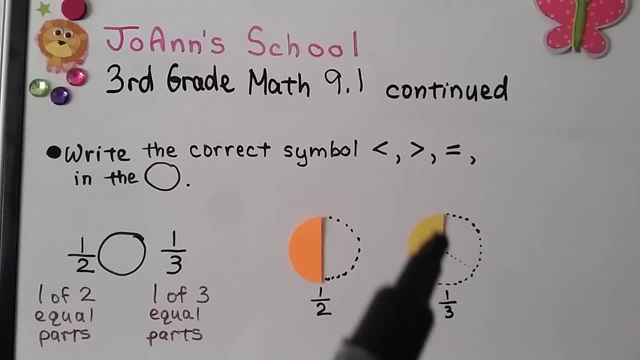 But when we have 1 of 3 equal parts, they're cut into smaller pieces, because now we have the same size circle, but it's in 3 pieces instead of 2 pieces, So we can see that 1 half is greater than 1 third. 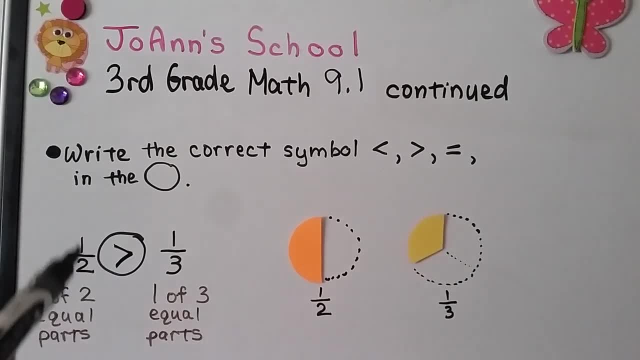 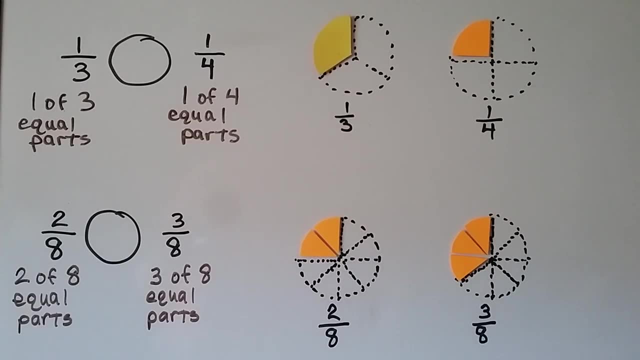 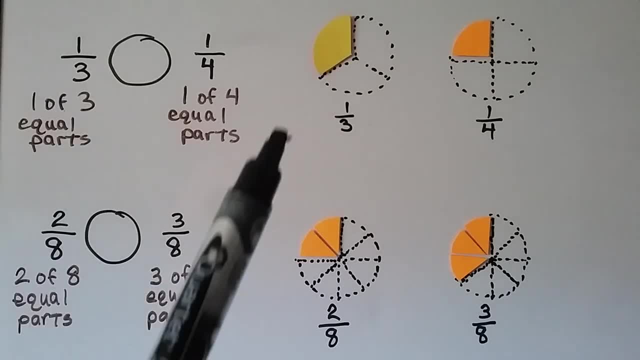 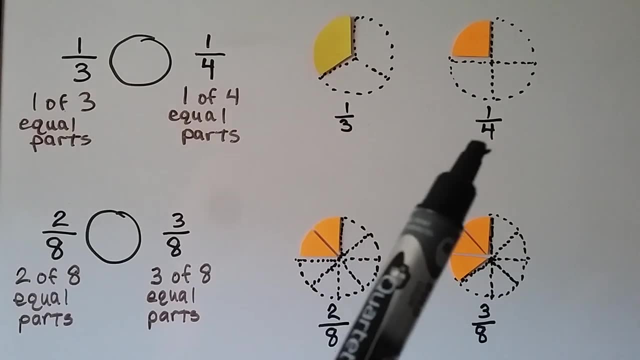 1. third is 1 of 3 equal parts. 1 fourth is 1 of 4 equal parts: 1 third means our circle is cut into 3 parts and we have 1 of them. 1 fourth means it's cut into 4 parts because the denominator is 4, and we have 1 of them. 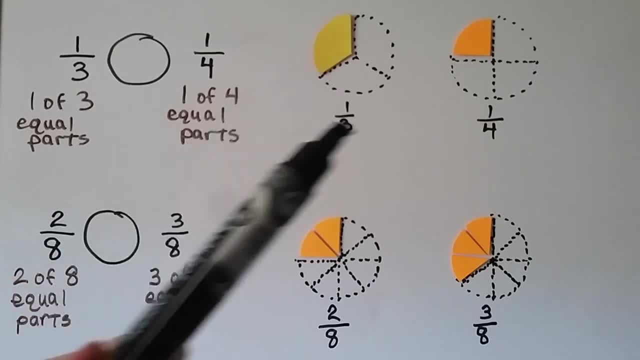 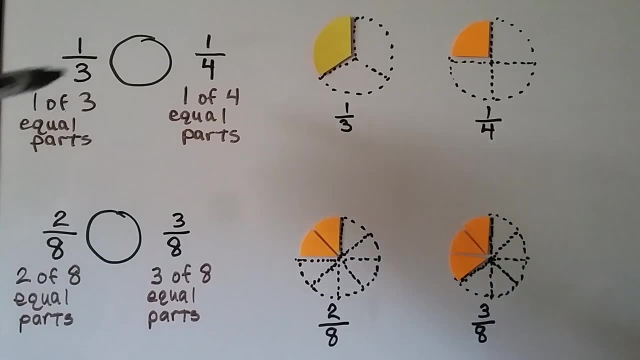 Can you see which one's larger We can see? 1 third Takes up more space, So one-third is greater than one-fourth. Take a look at this one. These have the same denominator. This is two-eighths, or two of eight equal parts. 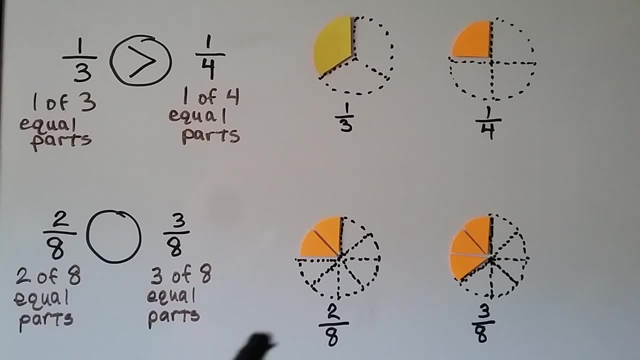 This is three-eighths or three of eight equal parts. So both circles are cut into eighths. This one has two equal parts, This one has three. We can see that two-eighths is less than three-eighths. 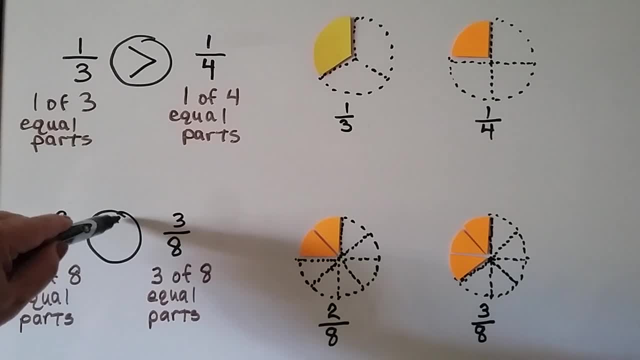 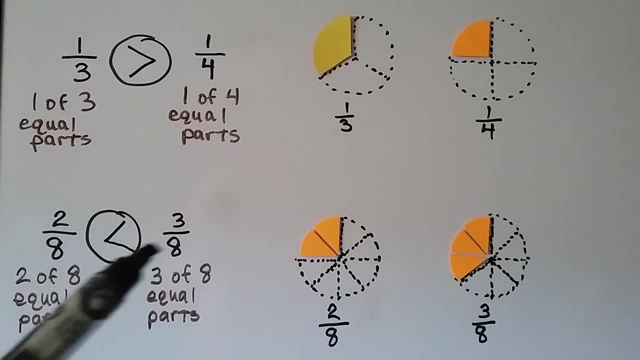 It takes up less area. It takes up less space, doesn't it? So we're gonna put the little side towards the two-eighths and the big side towards the three-eighths, because two-eighths is less than three-eighths. 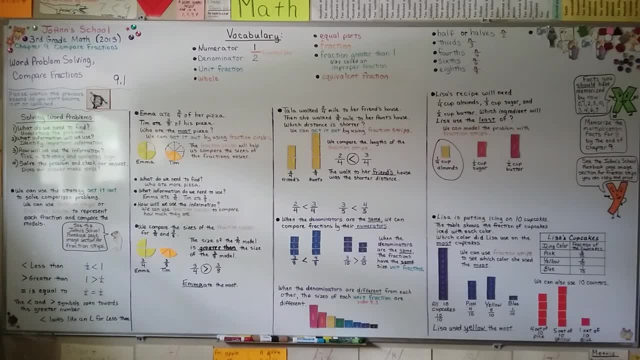 Make sure, when you're using the less than greater than symbol, that you're using it facing the correct direction. The big opening faces the larger number. We're gonna talk about how to compare fractions with the same denominator some more in our next lesson 9.2, and I hope I'll see you there.